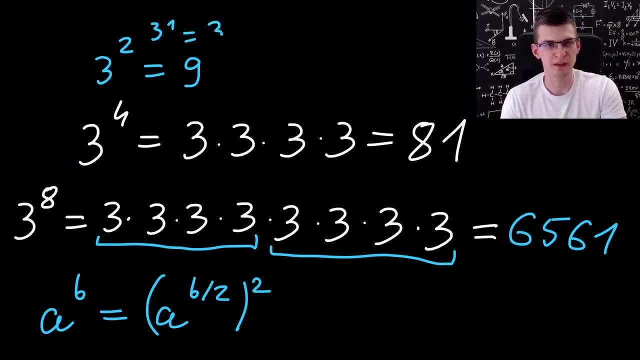 How to compute 3 to second power. Of course it's 3 to 1 square. If you are given this number, then you can quickly compute 3 to 16th, because it's just this times itself and that's it. This is already working code, at least for b being power of 2.. 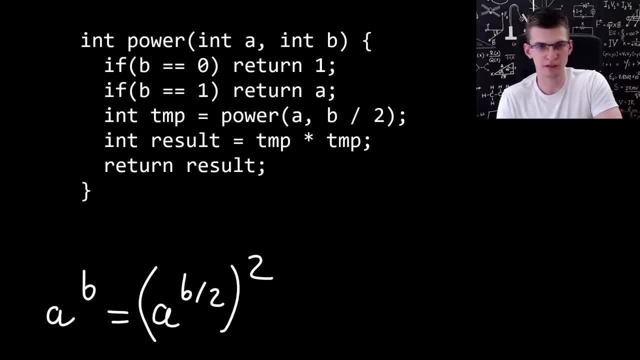 Where if you want 0th power, then for every a it is 1.. First power is just a. later we will see that this if is really unnecessary, And otherwise you recursively compute a to b over 2 and multiply by itself, just using this formula from below. 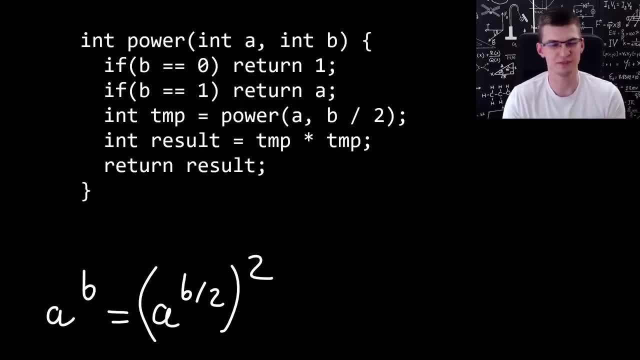 This does not really work for odd numbers and generally for numbers that are not powers of 2.. If I need 3 to 11th, then my code here will try to compute 3 to fifth power, because b over 2 rounds down towards 0 and 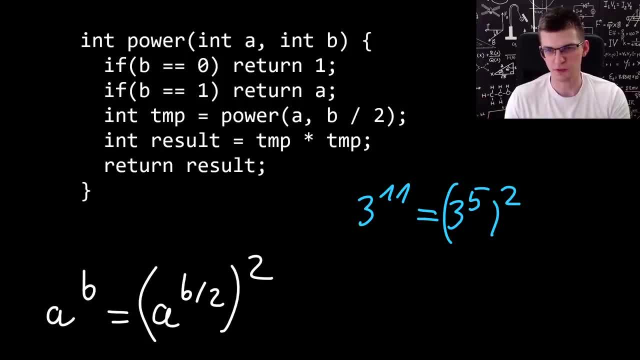 square. and let's see what is missing in this formula: 3 to 5 square, it's 3 to 10th power. I need to multiply by 3 and then it works. As always about recursion, it's enough to think in my current run of recursion what smaller run I need in order to compute the answer correctly. If this answer is true, then I will use this simply. If this answer is true, then I will use this simply. If this answer is correct, then I will use this simply. If this answer is incorrect, then I will use this systematically. If this answer is correct, then I will smooth that. êtes la. I will do the same. If this answer is incorrect, then I will get two more. 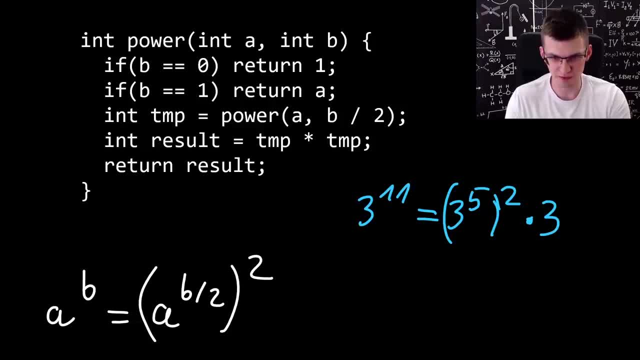 computed correctly for that other run of recursion, then my value will be computed correctly as well. I don't need to think about it and go deeper and yeah, let's just fix this code like that. After computing result, I have this: 3 to 5. 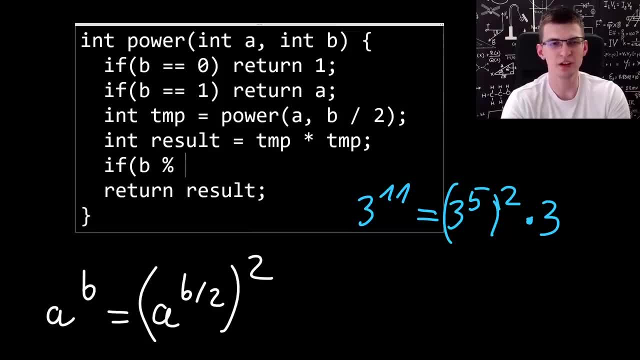 square. I say: if b is odd, then multiply the result by a and it turns out that this is already a working code for our problem of binary explanation. you can use it and this if turns out unnecessary. If you have 3 to first power and you 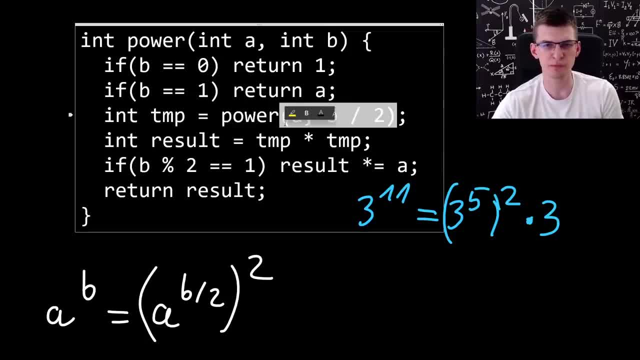 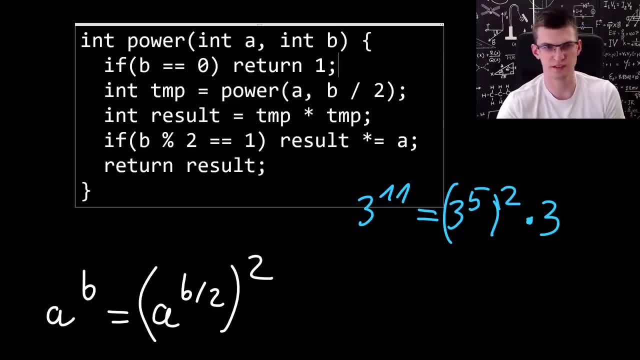 analyze this piece of code. it will run 3 to 0 of power and then multiply a result by itself, so it will be 1 times a, anyway a and this is not really necessary. We can analyze this run further. We need 3 to 5 and it will be. 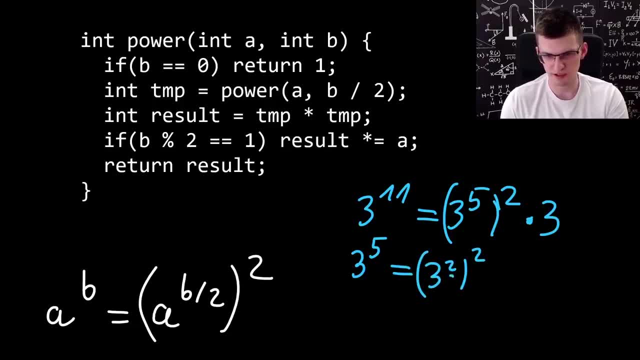 computed as 3 to 0.. 3 to second power square. second is because it's b over 2, b was 5 a moment ago and we need to multiply it by 3, then we need this recursively. 3 to second power is 3 to 1 square. this computed recursively. then we take square in this. 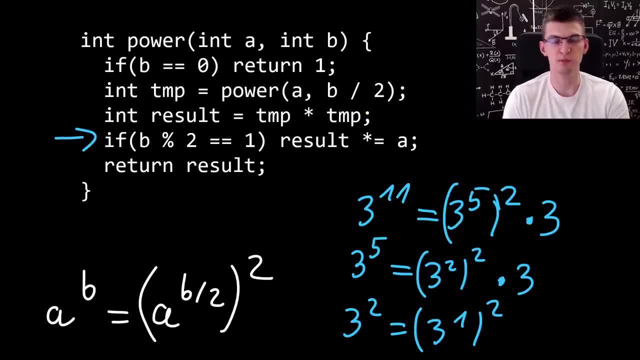 line. and this does not happen. If b is even, then the formula from below, this formula exactly works for even b, otherwise we need to fix it. We need to fix it by saying times a if b is odd, and finally 3 to 1. we either can have an: 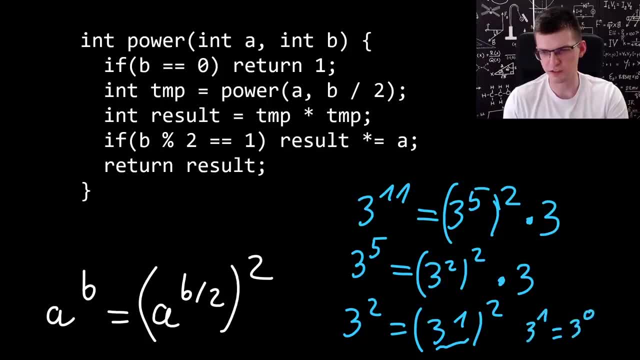 if, or we can say that 3 to 1 is 3 to 0, square times 3 also, it works correctly. One more look at the code to make sure we understand what it does. This is some base case. a to 0 is 1 unless a is 0, but that's a stupid case. Let's say that a is not 0.. 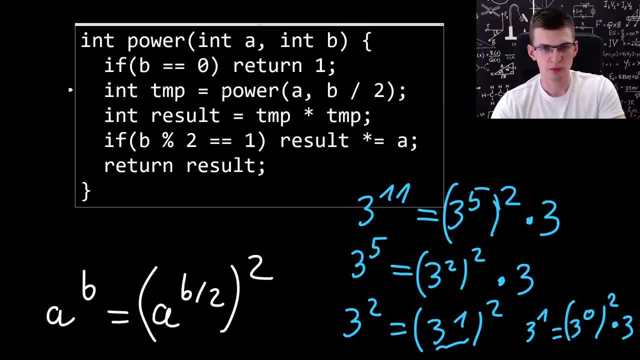 Let's say that a is not 0. We compute recursively that power a to b over 2 and we save it as some variable. You cannot say this times itself and again, type power of blah blah, because then it will be recursively run again. You don't want that, because you. 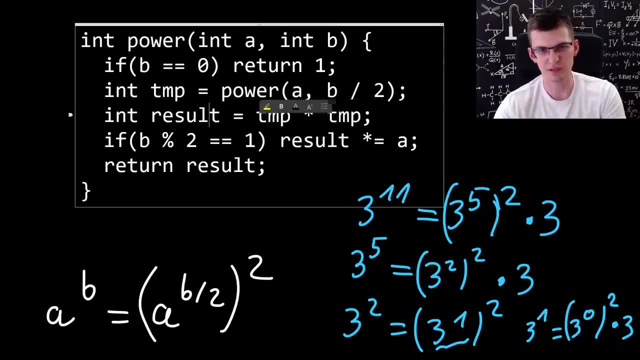 get worse complexity. tmp times tmp is result and finally, if b is odd, then fix that result. That's it. If a and b are not small values, then obviously this is C++. we can have some overflows if we use int And most of the time you will want this to be taken: modulo some prime value, for example. 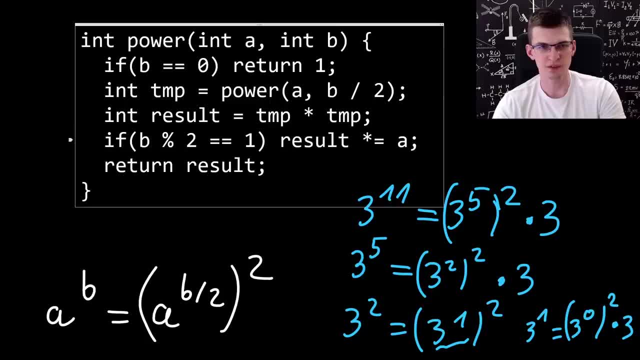 and there was previous video about what it means. Most of the time, if you want to compute like 50 to power 50, you don't really want to get that huge number. but if you are in Python, of course you can compute that and it will just work. Otherwise, remember to take 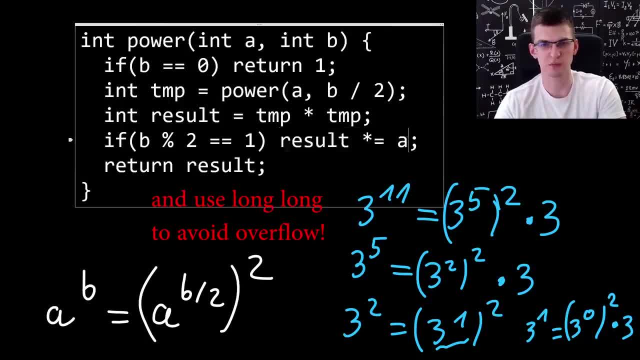 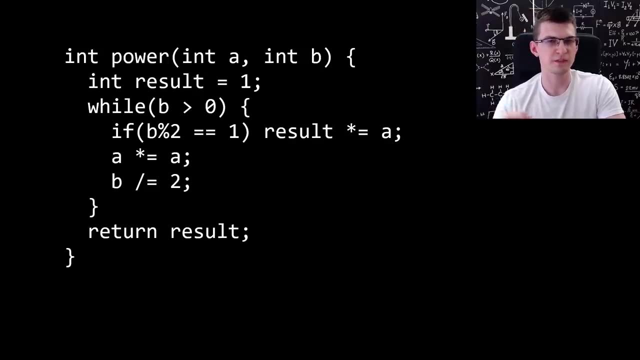 this product modulo m, and to take this product modulo m as well. While this code is perfectly fine, I don't use it Because Iterative programs are faster than recursive ones, and this is code I use during programming competitions. It's iterative version of the same thing, where I finish when b is equal. 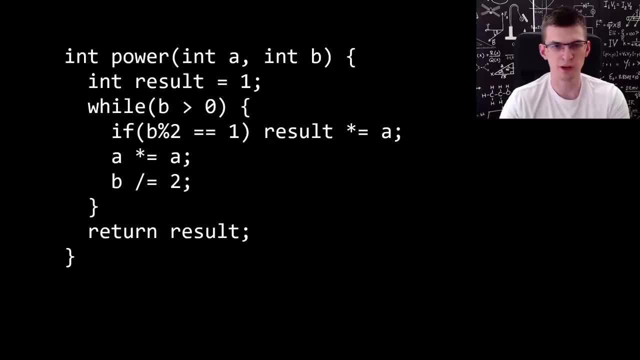 0. the same happened here in the first line. While b is greater than 0, I update result in some way. If b is odd, modulo 2 is 1, then multiply result by a and otherwise we have something strange. multiply a by itself. 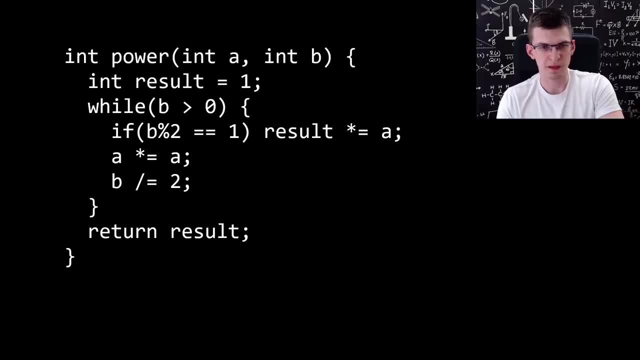 Let's think what this means. and an example of 3 to a: 11th maybe. Because, well, first, if is b odd, b is equal 11, so sure it is odd. result is already multiplied by a. So we say that result is 3 times and there will be something more. Now we increase a Instead of 3. now 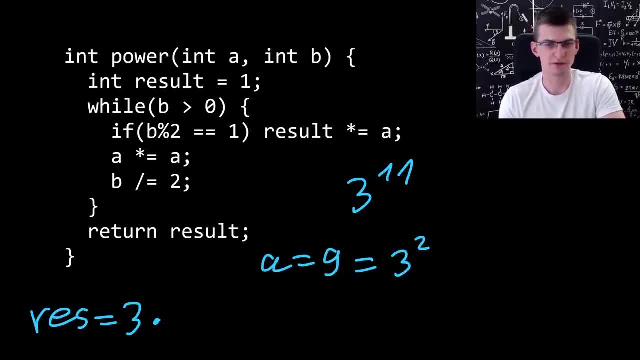 a becomes 9.. It is, let's remember, 3 squared. So we increase a Instead of 3. now a becomes 9.. It is, let's remember, 3 squared. We divide b by 2.. So now we want to just come to compute 3 to 5. fifth power: 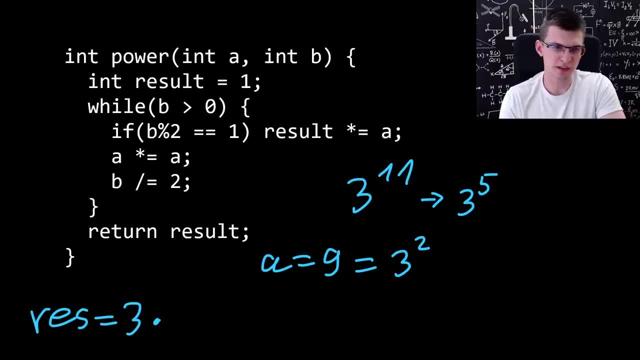 This is odd. So in the next iteration of the while loop, this if is triggered and we multiply result by a- This time a is 9 or 3 squared. Then we multiply a by itself, a becomes 81, which is equal to 3 to fourth power. Divide b by. 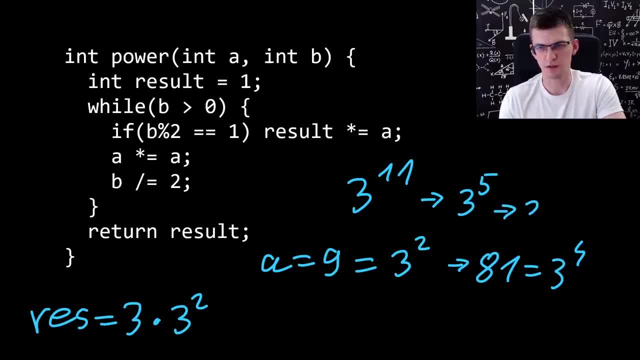 2.. So b is now we need this. b is now 2.. This is not odd, and we don't update the answer or result. We just multiply a by itself. Now it becomes that big number, 6, 5, 6, 1, equal to. 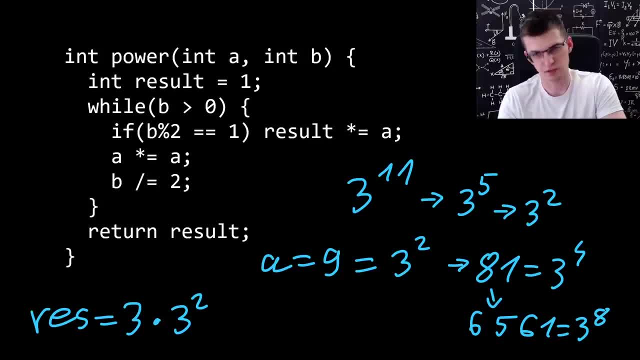 3 to 8th power. Divide b, b becomes 1.. We need 3 to first power. And now b is odd. for the last time We multiply result by a. No matter what happens later, result will not be changed anymore. 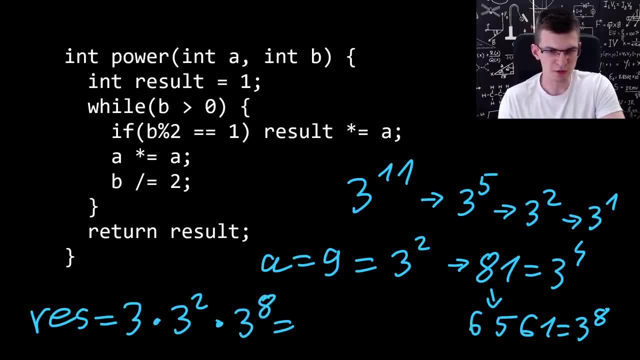 The last thing was this difference And magically we got a correct answer, because 3 to a- let's say 3 to x- times 3 to y is 3 to x plus y. This is equal to 3 to 11.. But was that a coincidence? We need to really understand why this is equivalent to recursive. 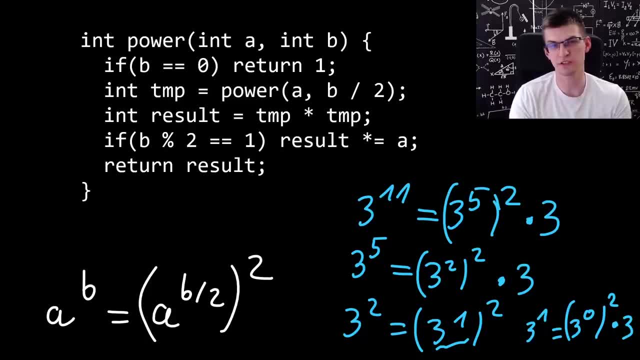 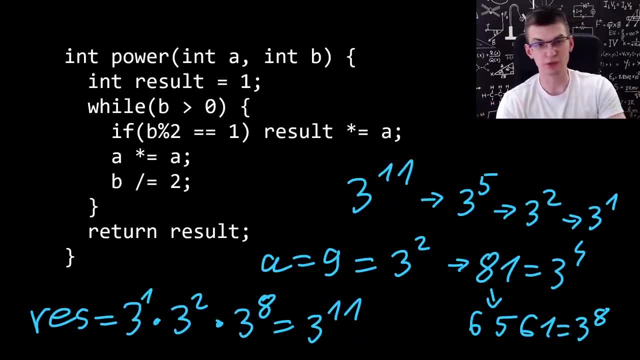 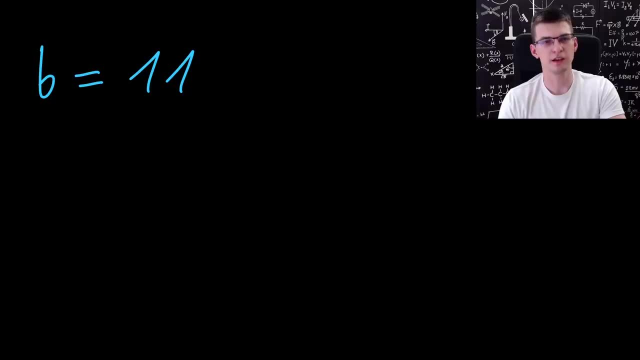 version, even though recursive sounds. recursive version seems more Reasonable, Intuitive And I think for better understanding of what really happened here we need to look at binary representation of number b. For 11, it is what 8 plus 2 plus 1.. So in binary system this is b. Our 11 is equal to 1, 0, 1, 1 in binary system And recursive. 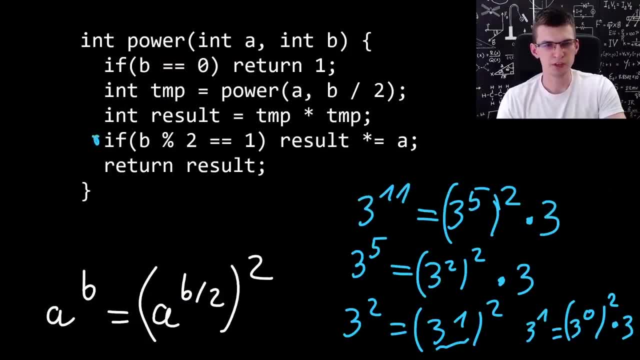 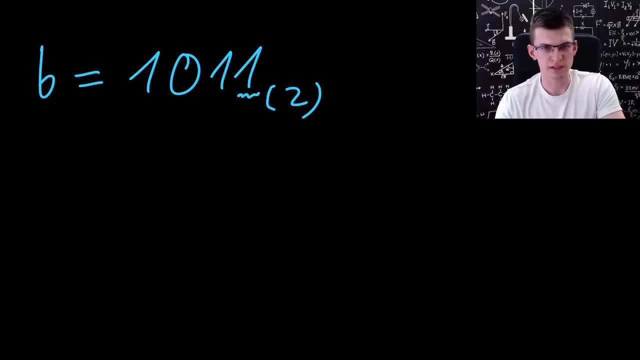 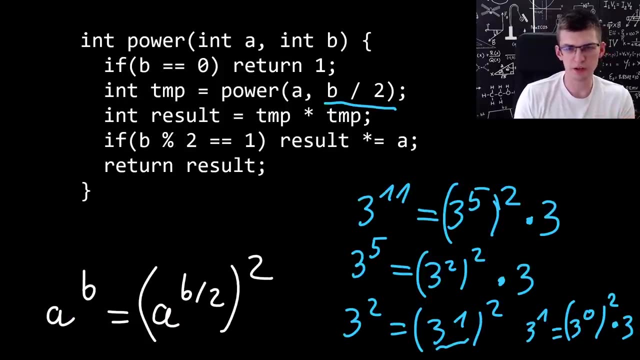 function This one. It multiplied result by a Only if b is odd. So that depends on this last bit. If this is 1, then multiply answer by a. Then when we take here b over 2. We get rid of the last bit in binary representation. 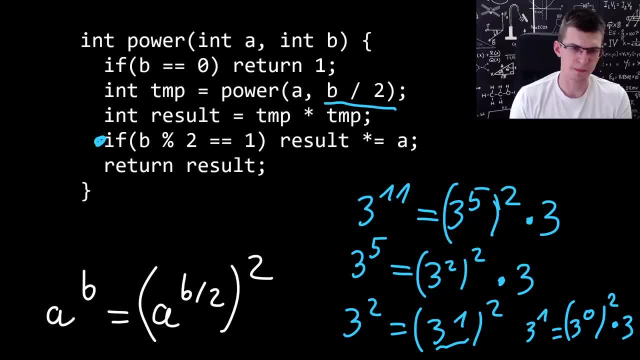 And here we get again: result multiplied by a Only if b is odd. So if that second last bit is 1. Then multiply result by a. But that happens recursively And the main difference, The main run of this, After running this recursively, for b equal to 5. It computed its value square. 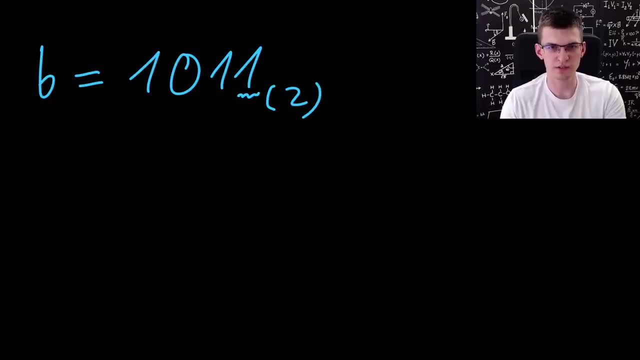 b equal to this Run recursively. that smaller thing Took some answer from that and took it then square. So if there was result multiplied by a Coming from this bit, Then later this result from that was squared. So we got From that a square. 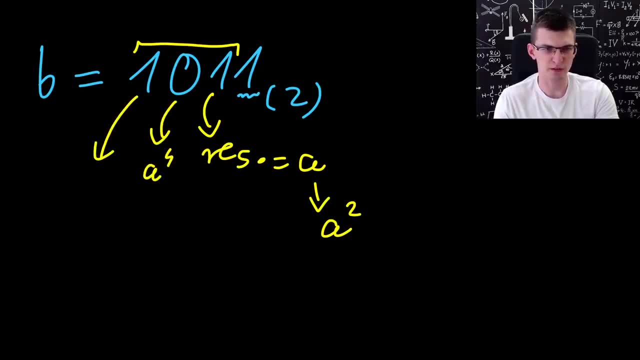 Similarly, this contributes as a to 4th power And a to 8th power, And this is alternative interpretation of both recursive and iterative solutions- That every number, Every power of a And for the whole time we work with a equal to 3, for 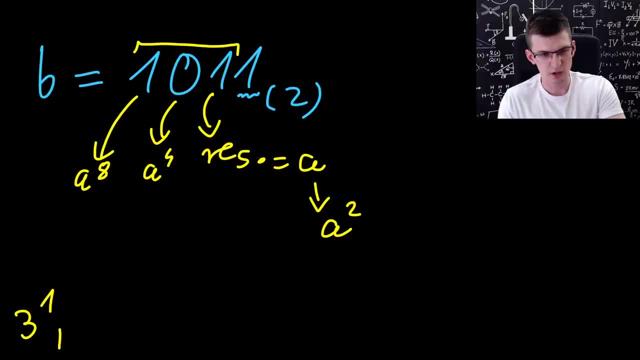 simplicity. The idea is that those can be computed efficiently in logarithmic complexity, And it doesn't matter if It happens recursively or iteratively. In some way you can compute those numbers. And now, whenever You're asked about 3 to some power, Let's work with 3 to 22.. 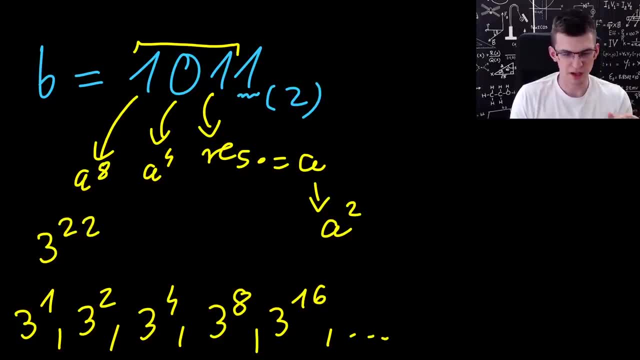 It is. I claim it is product of those powers of squares, Well, powers of, with exponent being power of 2.. 3 to 22, it is equal to 3 to 16 plus 8, not plus 4 plus 2.. So it will. 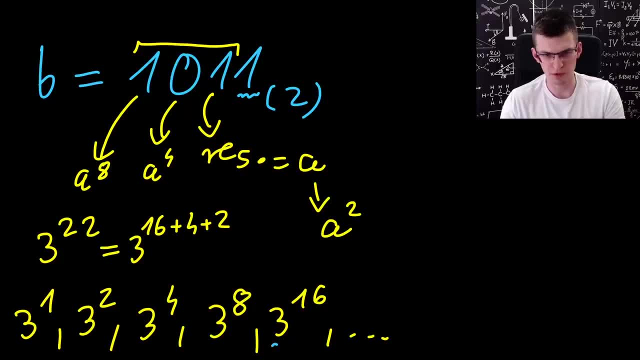 So it will be equal, maybe with blue 3 to 16th times 3 to 4th times 3 to 2nd power, and you can even put those powers in some array and then take a binary representation of b and then you will know which numbers you will need to multiply from this array of special 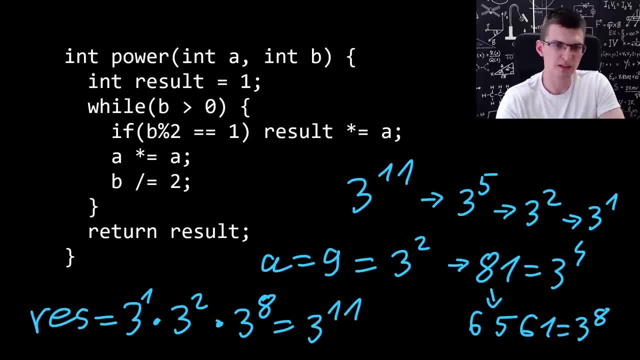 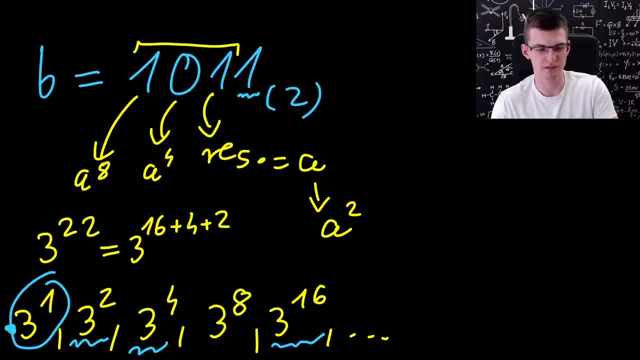 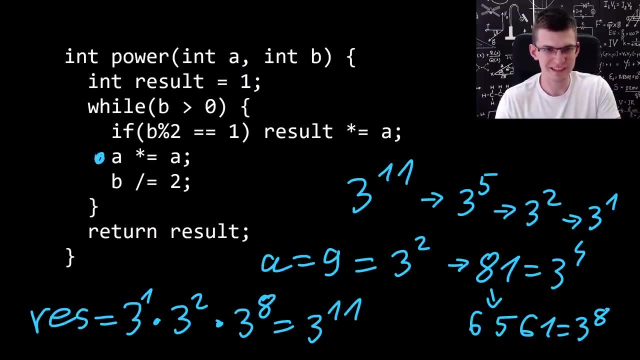 powers of 3 that you computed, But instead this iterative solution will do that for you. It will first know 3 to first power, so just a, and then it will compute a square, that thing square, and so on. This line computes 3 to 2nd, 3 to 4,, 3 to 8. 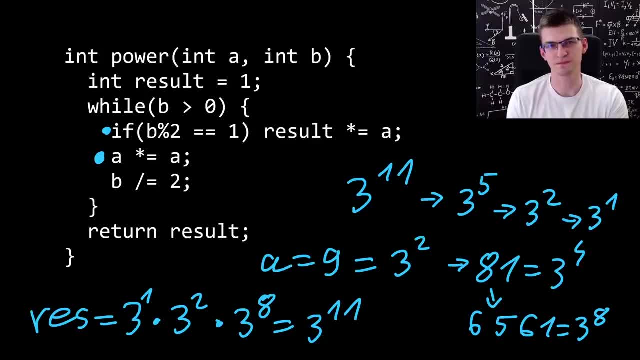 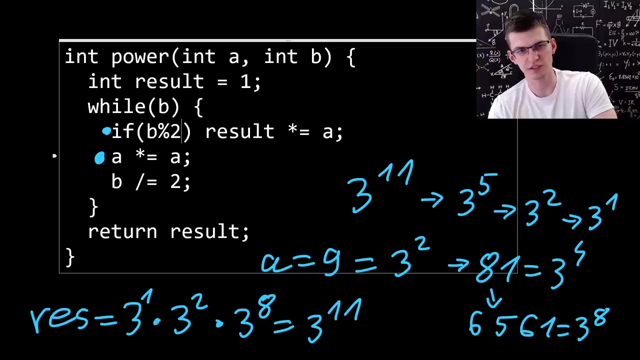 and this line just takes the last bit of b. So that's really understanding of iterative solution and, as I said, in general iterative solutions are faster than recursive versions. so I recommend this code In C++. you can also type it like that because by default if conditions while conditions, they check if integer is non-zero. 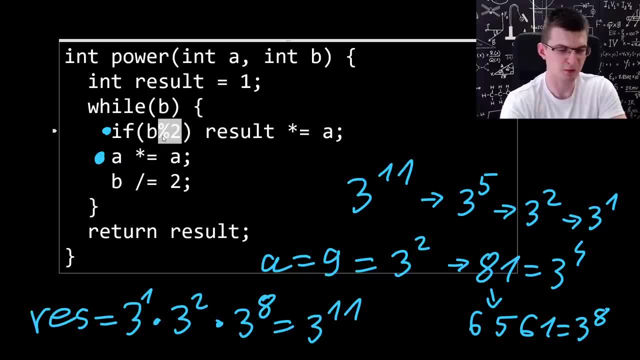 So this works as well. Some people here type n to n. if you will see in somebody's code then it's equivalent. I prefer modulo 2 because for me as a human it's easier to think about remainders rather than bits. but sure, And 1 will take a look at the last bit. 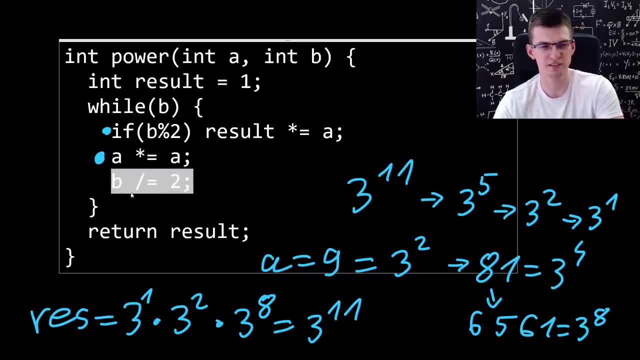 so that's also valid. Again, this can also be written in some alternative format, like shift b by 1, but what's the point, And most of the time this will be taken modulo. so result: times a modulo some m, and this thing as well: a is times a modulo m. 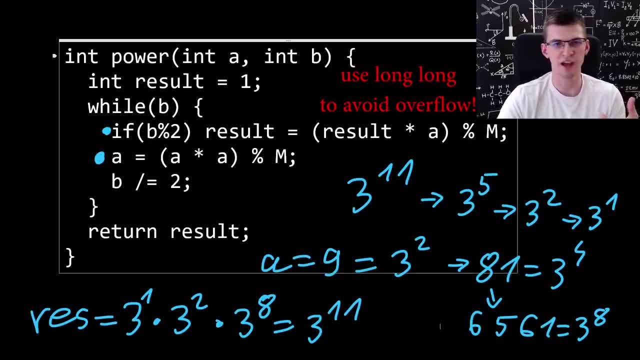 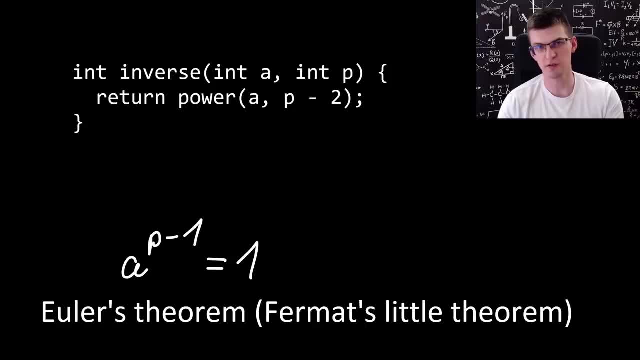 That's really code I would use if I wanted to compute a to b power modulo m in logarithmic time. As I already mentioned in the previous video, power of a number is something we need to divide by this number or to compute modular inverse. There is some smart theorem: Euler's theorem. 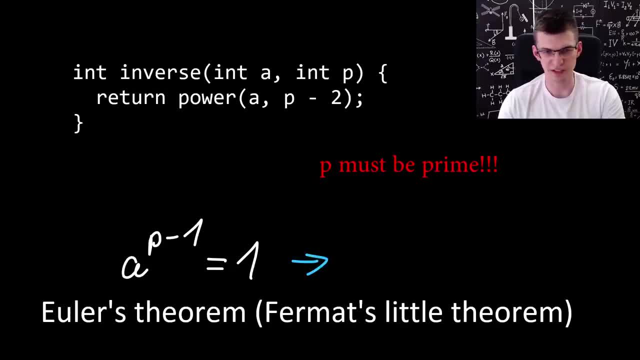 which states exactly this. and from that, if we divide both sides by a, we get a to p minus 2 is equal to inverse of a, 1 over a In this field, in this, let's say, world of numbers, modulo p. and then this is code we need. where power is our function written here, Everything happens modulo. 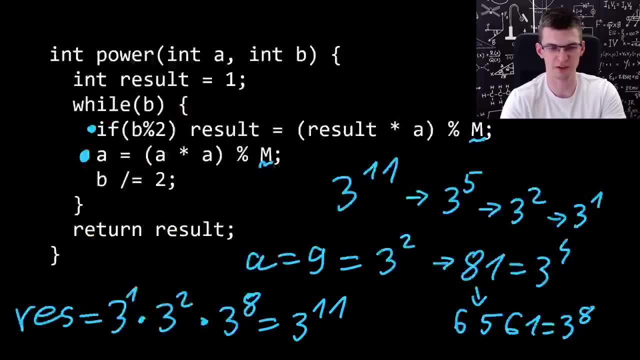 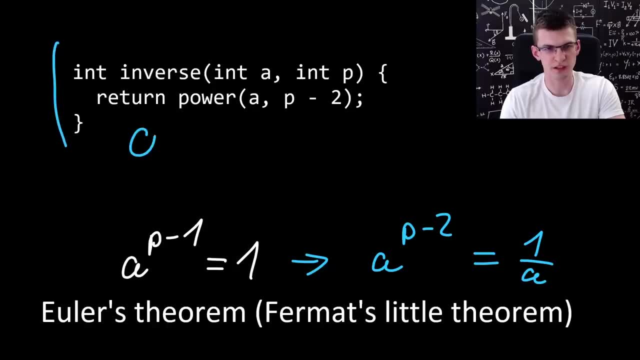 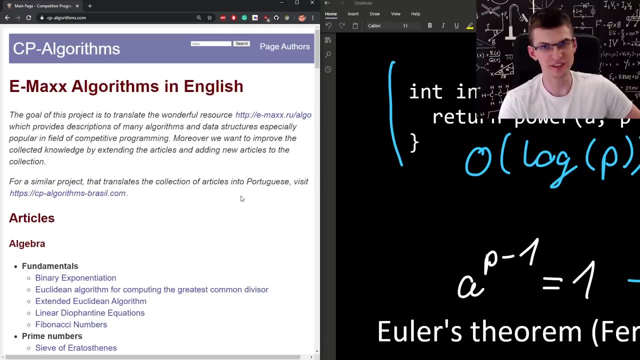 well, I used. this should be p, this should be p. if, of course, you want to use variable p And that will work. modular inverse like that can be computed in complexity logarithm of p. If you want to read more advanced stuff, I strongly, strongly recommend. 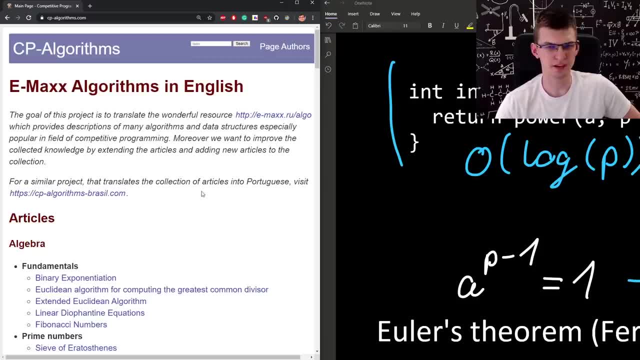 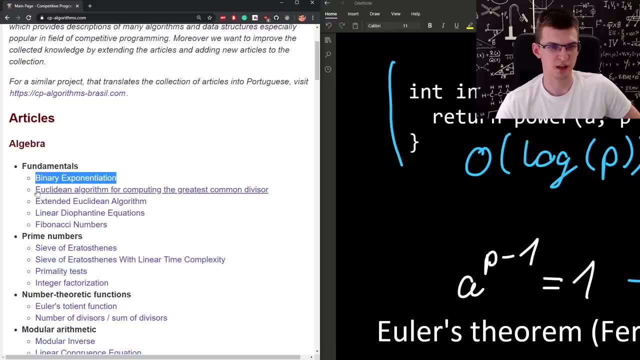 the website cpalgorytmscom. It has materials mainly on advanced and maybe intermediate algorithms, but at the beginning there is, for example, binary explanation, also then Euclidean algorithm in its extended version. They can be used as well to compute modular inverse. and then there are some important things about prime numbers, number theoretic. 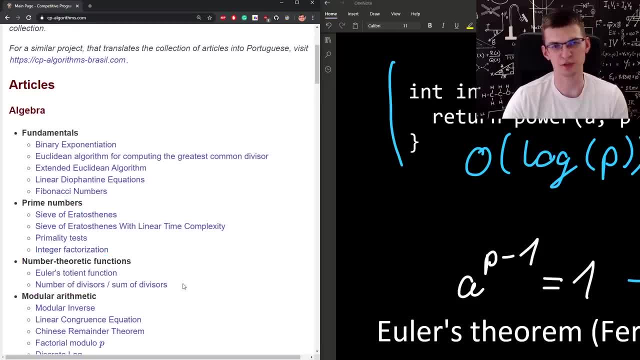 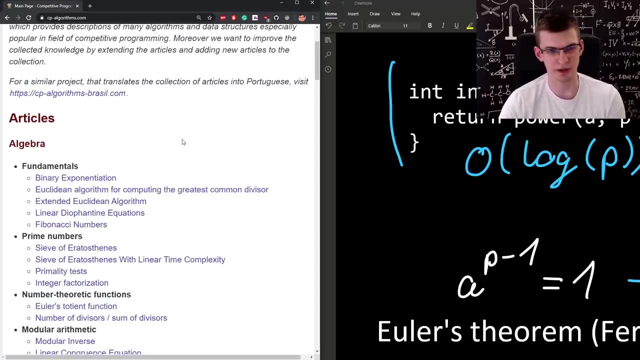 functions. This is important as well to understand how to compute the number number of divisors. to sum them up, I think this is needed to compute modular inverse for non prime numbers. it's cp-algorithmscom. actually it's translated from Russian and there it's just Emacs. so do check out that, oh. 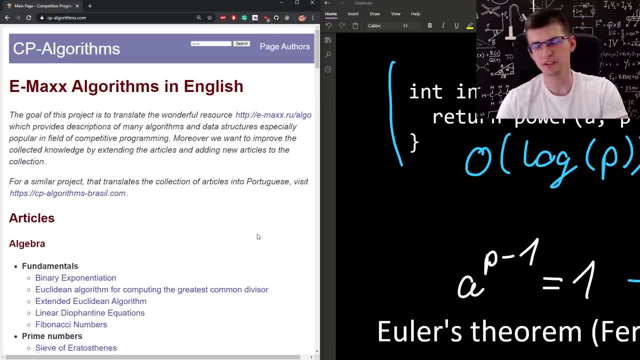 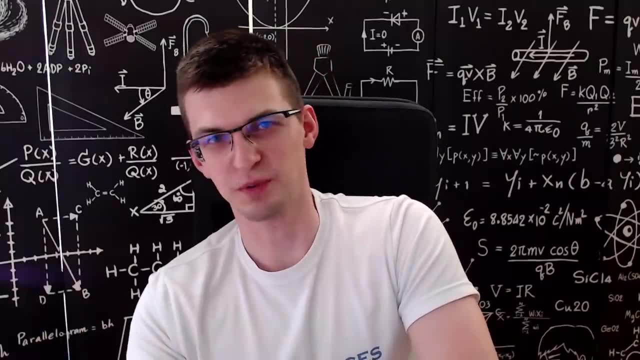 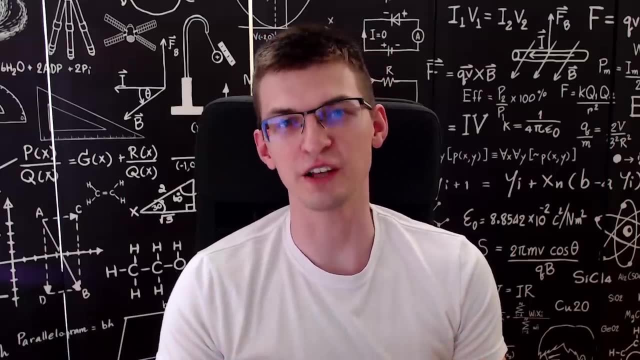 actually there's even an article on modular inverse link is also in the description. our next lesson, the next video, will be about something more advanced: matrix explanation- the thing we learned today but applied to matrices, and you don't really need to right now understand matrices. I will explain that. 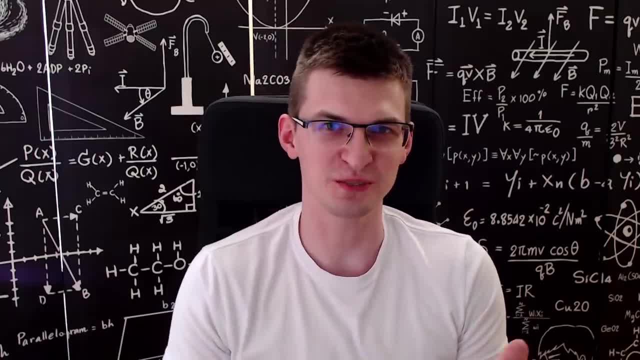 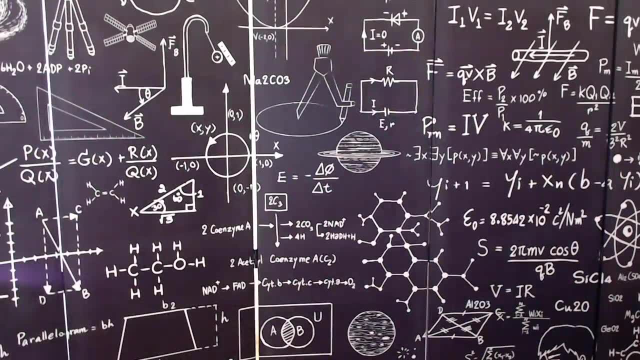 to you, so be sure to subscribe to the channel. turn on notifications. if you liked the video, then leave a like and I'll see you in the next one. bye, thanks for watching you.